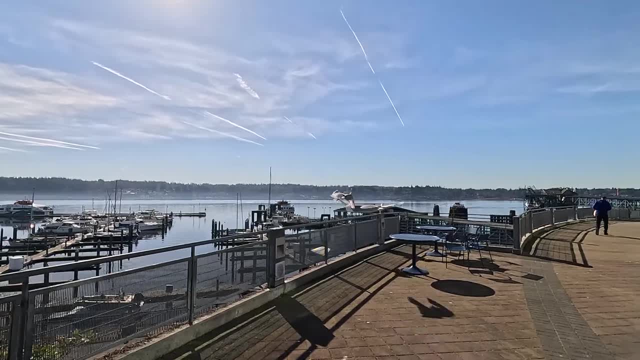 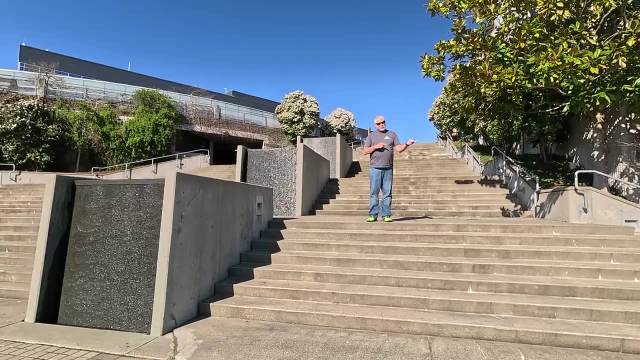 The Turner Joy is right down this way. It used to be. the old Missouri battleship was there. It went to Oahu. They brought in the Turner Joy Excellent tour museum, naval history stuff. Really a cool place to go see. 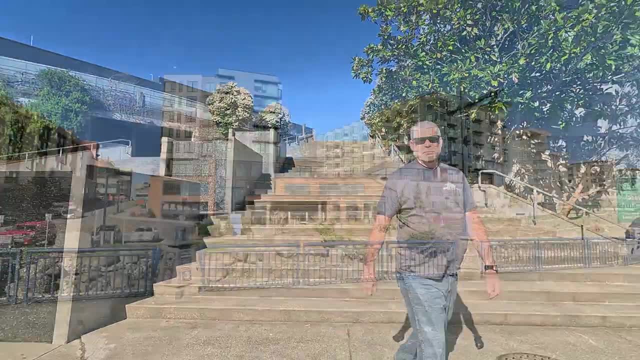 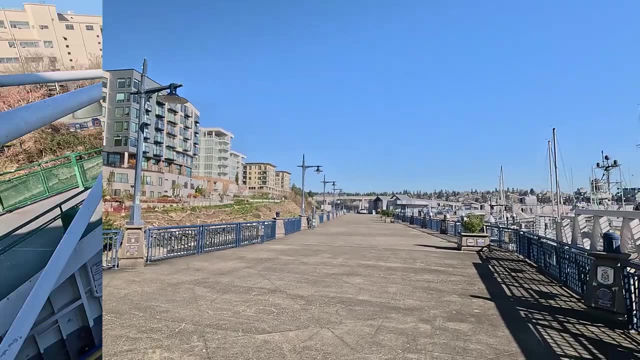 We're going to jump on the ferry here in just a couple minutes and head over to Pike Place. If you don't know where the ferry end goes, make sure to check out the site and the navigation app. Let's go, Let's go. 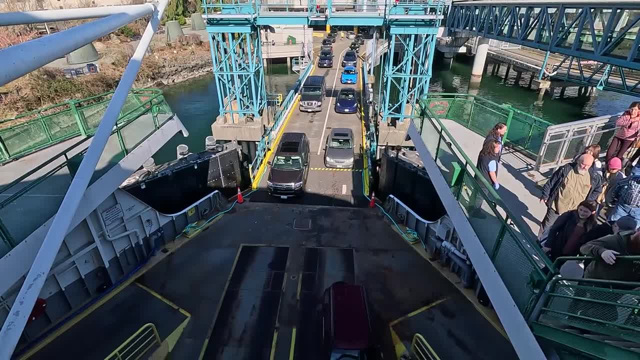 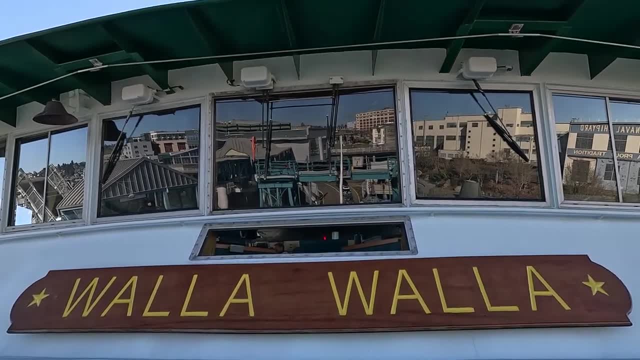 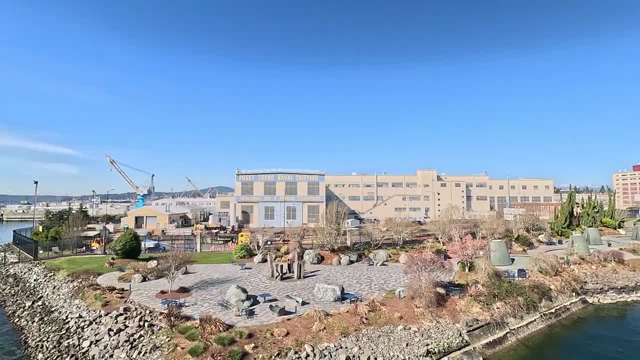 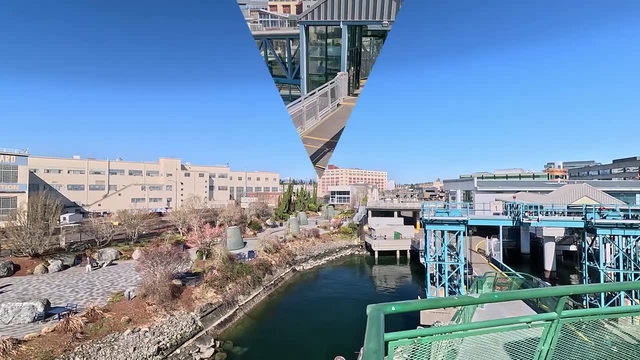 On the overhead passenger deck is the perfect viewpoint. If you drive on to the ferry, pay close attention to the deck crew for directions in which lane to drive in and where to park. Washington State has the largest ferry system in the United States, carrying approximately 23 million passengers a year. 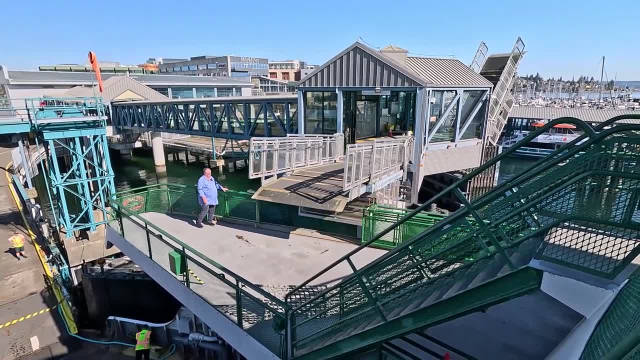 We were on the Walla Walla, which is a giant windsail cruise ship in the United States, And we're going to visit a small boat that's just west of the Puget Sound Naval Shipyard, which is a jumbo class ferry built in 1973 and rebuilt in 2003.. It can carry. 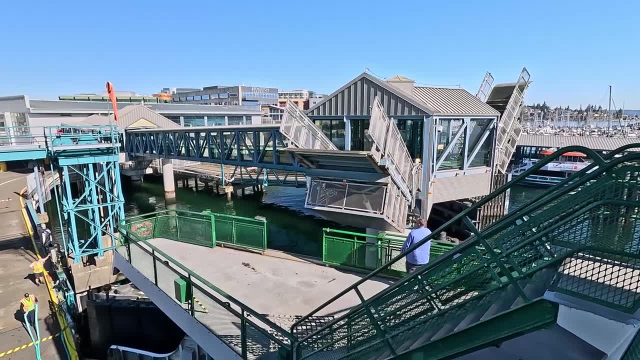 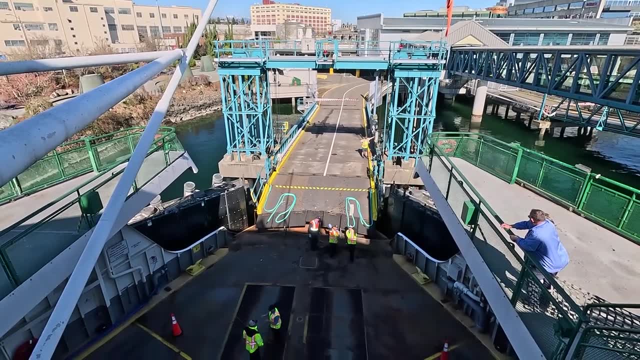 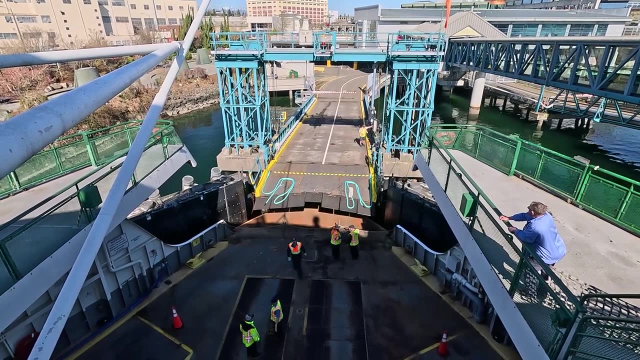 188 vehicles and 2,000 passengers per trip. The clearance on the autodeck is 15 feet 6 inches, so even if you're driving your RV, there's plenty of room for you to get on the boat Once all the passengers are loaded and the cars are. 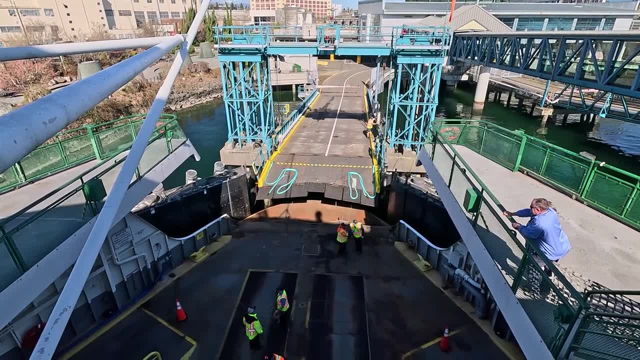 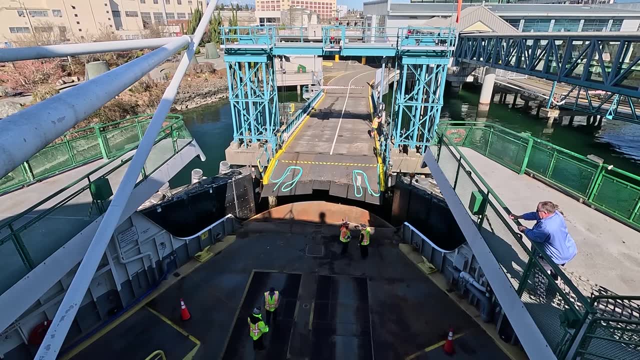 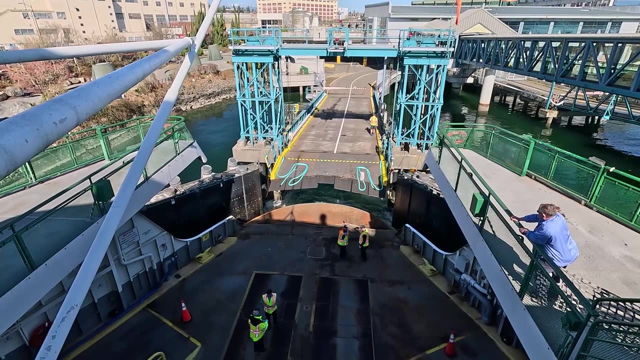 on. it's time to button up the ship and take off for the 60-minute crossing. During the crossing, you can visit the dining area, where you can purchase food and drinks, and even beer, up to 15 minutes before arrival at the other end of the trip. The fees for the Seattle Bremerton run are $17.90. 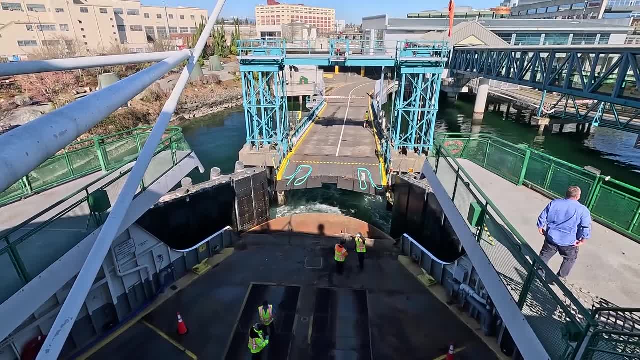 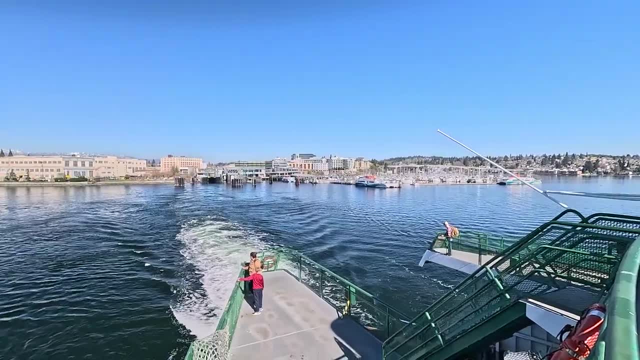 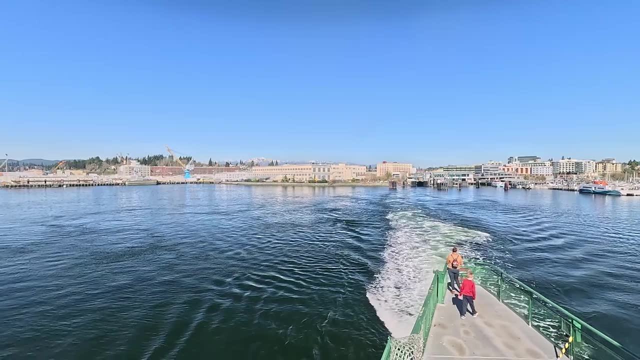 for car and drivers who pay both directions. Passengers pay westbound only and it's only $9.85 for the crossing, $18.00 and under for the cruise. Enter Ride2Boat for free, both directions. For more information, log onto WSDOTWAGOV. 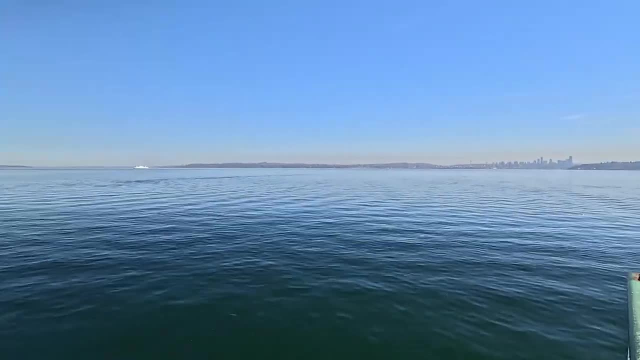 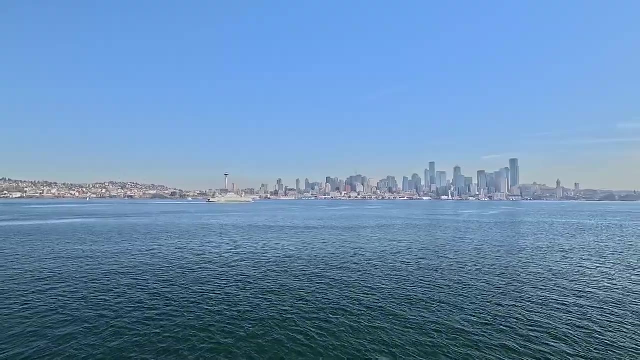 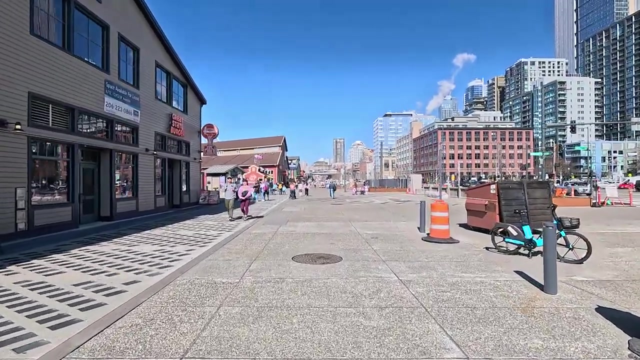 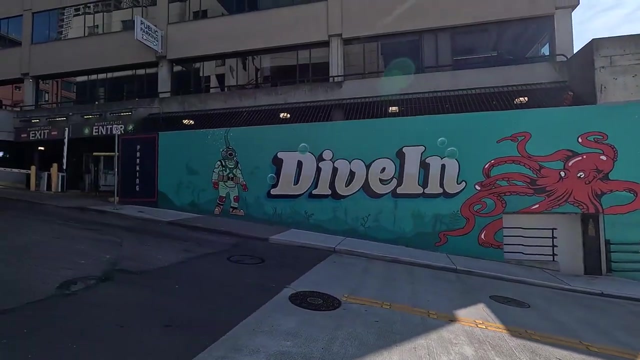 The Seattle waterfront has been under major renovation and construction since early 2019, when the viaduct was torn down and the downtown tunnel was opened. Parking is expensive but there's plenty of it downtown if you drive on, If you walk, walk up to the Pike Place Market and your first stop should 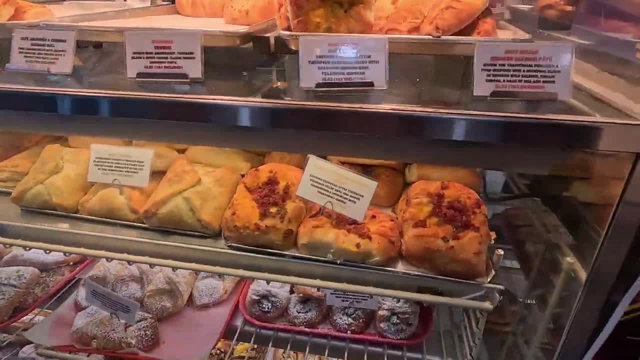 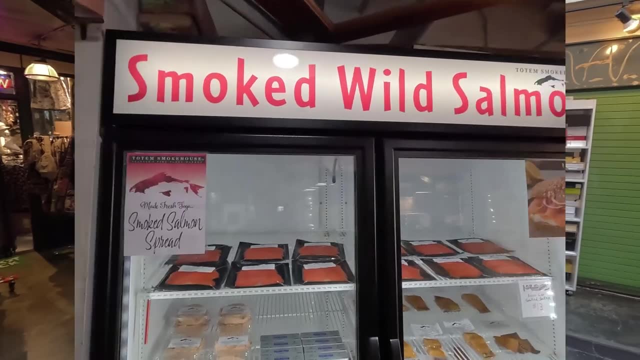 always be Poroshki Poroshki. Since opening a Pike Place Market in 1992, they brought a taste of Eastern Europe to locals and travelers alike. It is Seattle, so you never know what you're gonna find hidden away, but you can always find the best smoked salmon in the country. You can always pick up. 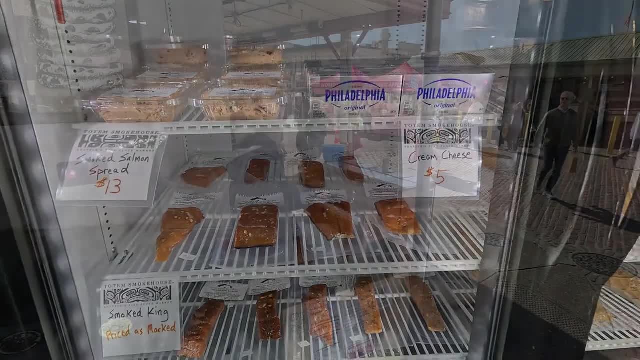 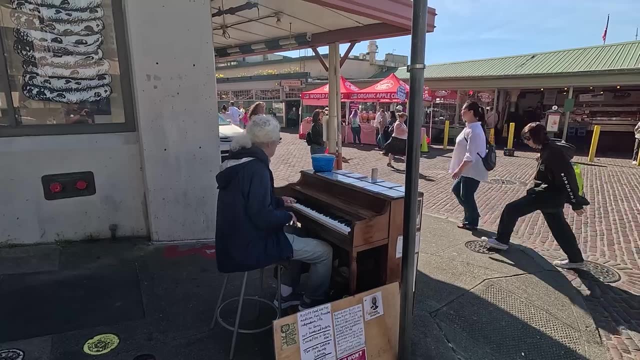 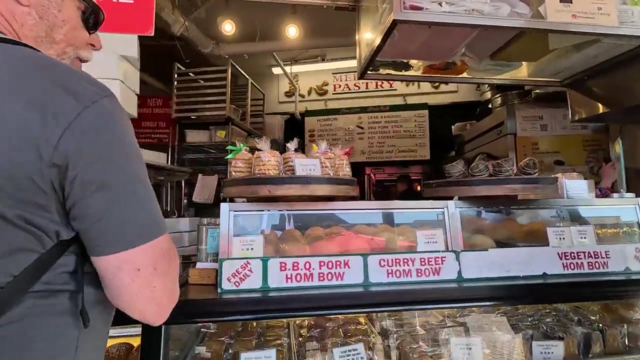 enough ingredients to make a good lunch and then stand around and watch the street performers. By about now you should be done with your Poroshki, and even the dogs know you have to try hamp out. Hi, can I get one barbecue pork, one curry beef and a beef? 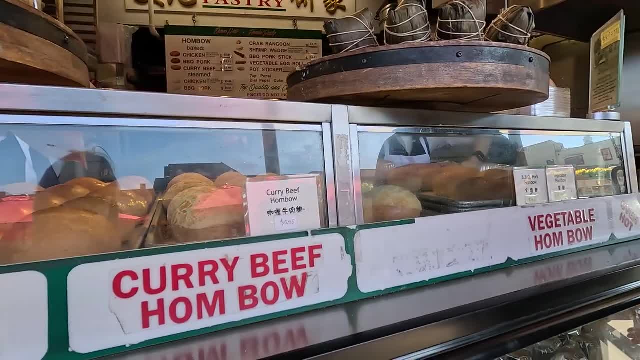 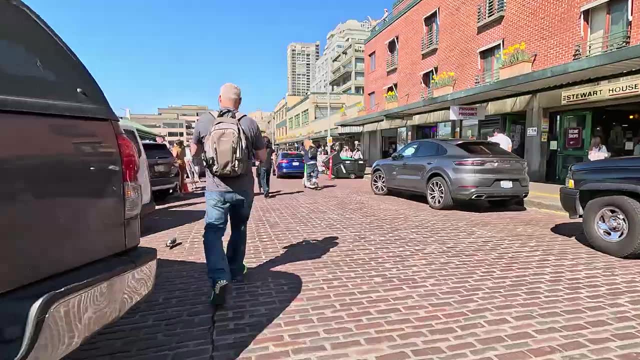 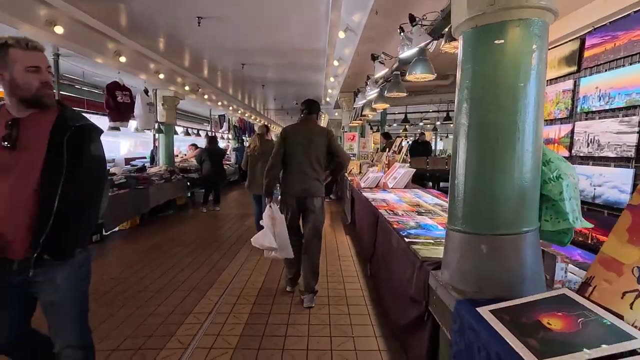 steamed bun. I have to admit, I have a craving for these little Taiwanese pillows of goodness. I think I probably like them almost as much as my kids, Casey and Megan do, and we always have to get some to share with her or take home. inside in the market stalls you'll find everything from t-shirts to 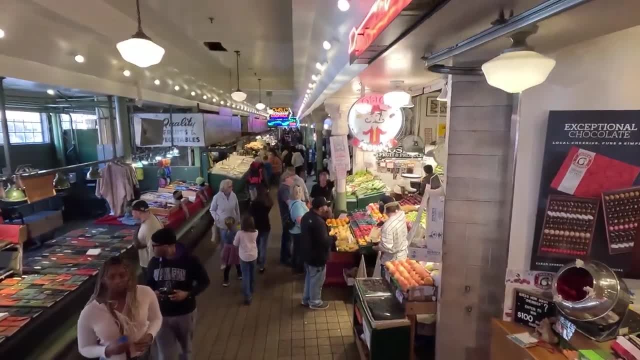 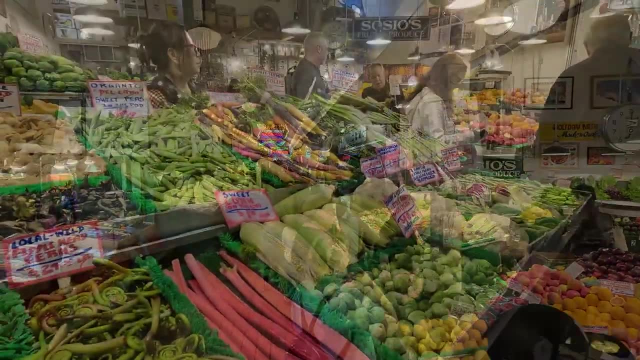 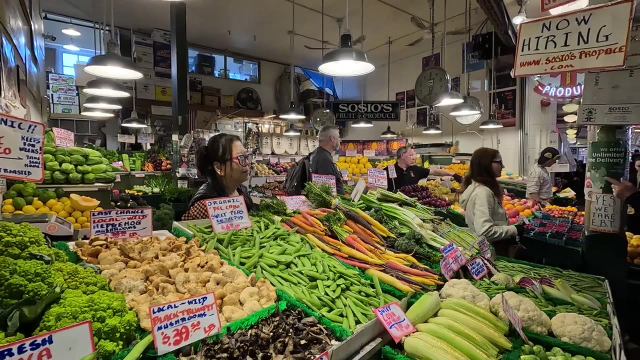 art, to jewelry, to flowers, but one place you don't want to miss is socio's produce. stop and see my friends there. grape, I do have kind of whether I basically the same thing in a seedless version now. so they call these green globes. it's the same thing, but they're, they're seedless, they're super crunchy. 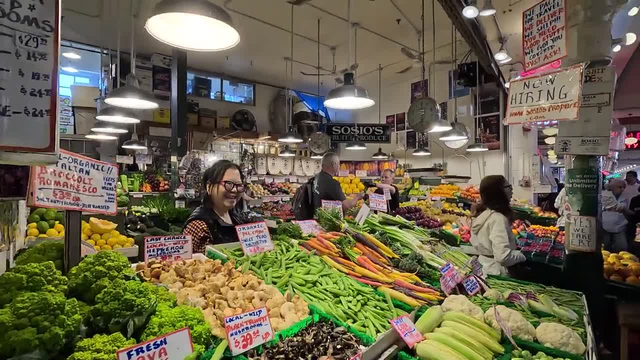 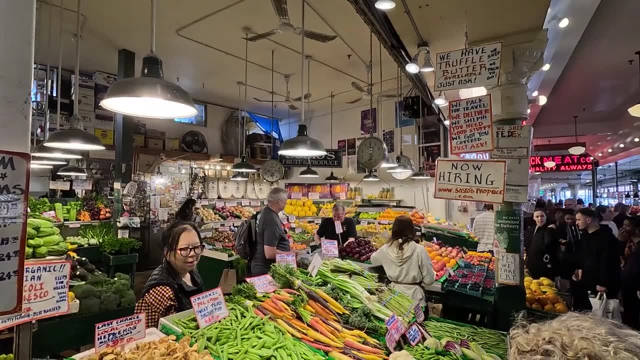 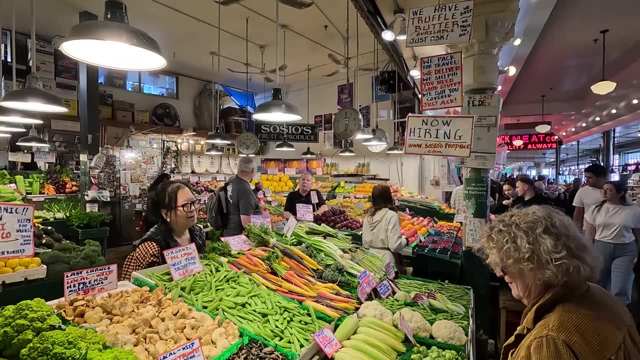 though really awesome. do you know? we're gonna have to have some of those go. yes, these are good. and then on the artichoke thing: the artichoke things- pretty interesting for people that have so see, people that grew up eating artichokes. in this country, for 200 years we only ate one variety of artichoke. it was a. it was. 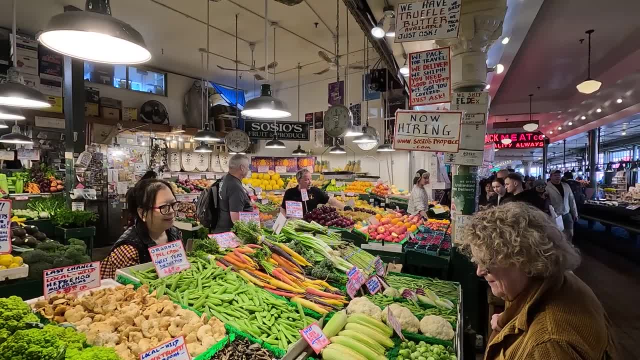 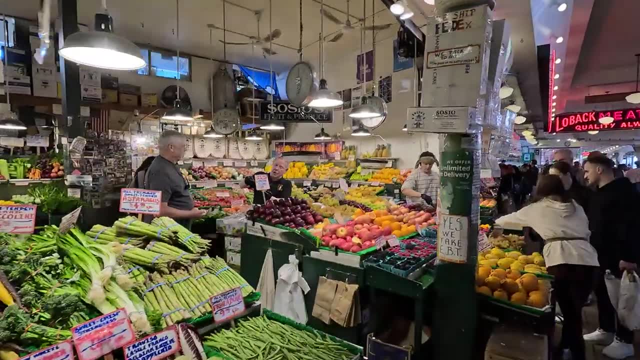 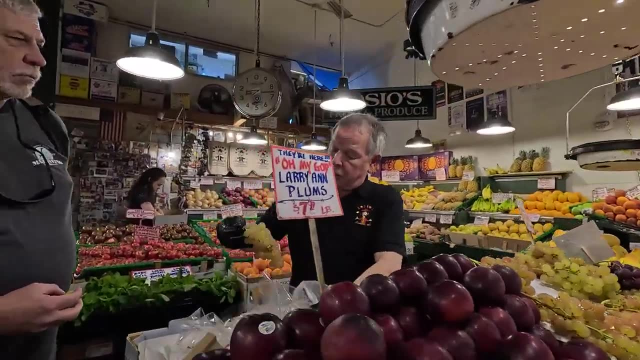 the original original artichoke from the Ellis Island cuttings- I mean, it's literally DNA of the original Ellis Island cuttings and thing is with them- is the only grew in one microclimate, only produced one crop a year. so about 30 years ago the industry developed a seed choke, one that could be planted. 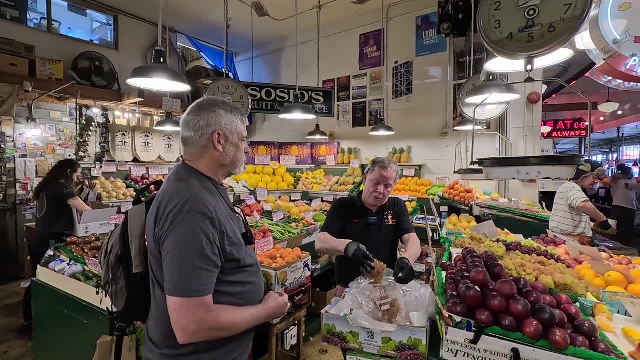 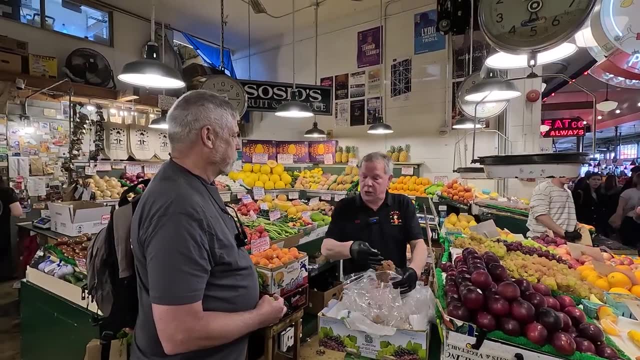 anywhere and produced three crops a year. the problem with that seed choke was it was three crops and crap, and so people that grew up eating artichokes, they all thought they, they all thought they're cooking them wrong or something. it's only boiling water, so we're not very smart in this. 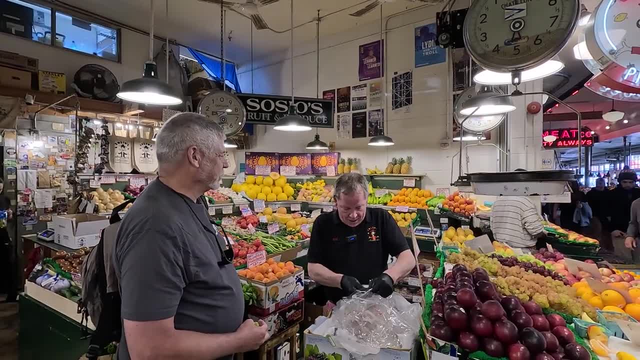 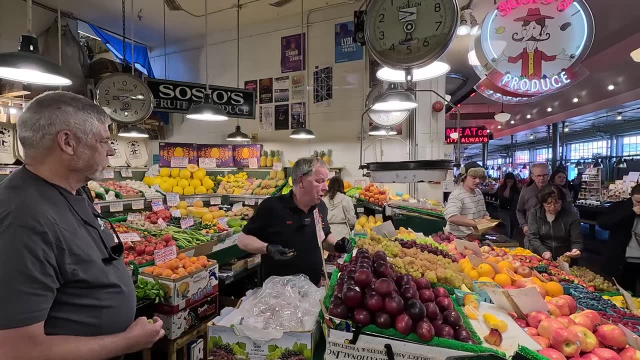 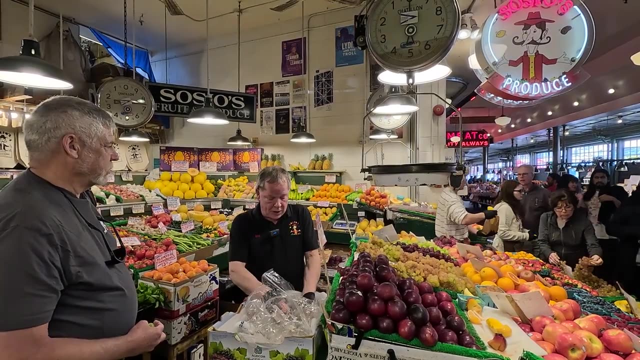 country. so we don't, we think there's something different and then we quite: yeah, but anyway. so, just through a convoluted series of events, only one guy kept any globe acreage and I'm his only retail outlet for the last 25 years. so people- that I mean my regulars, they all know about it. there's whole generations. 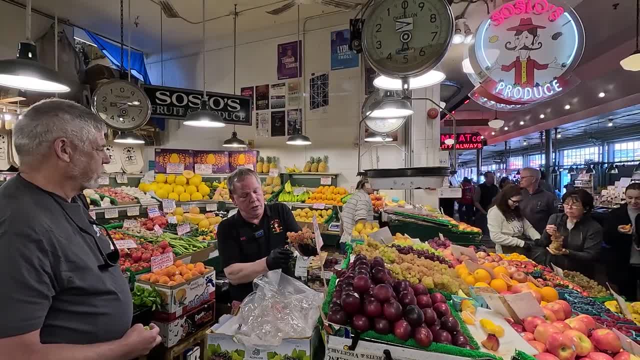 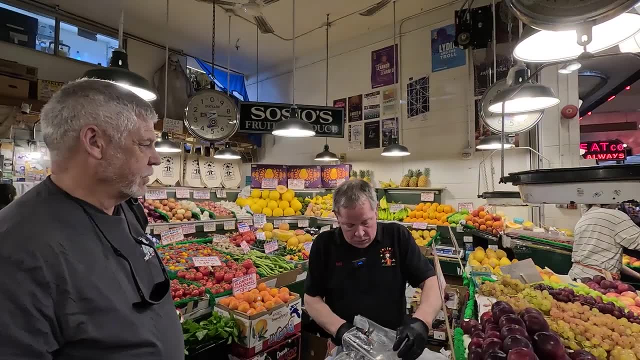 that have no idea what a real artichoke tastes like in this content in this country, you know. so people think they're just like. like I said, they think they're wrong. but so and it's, it's our, it's our deal. in the spring we can never get all. 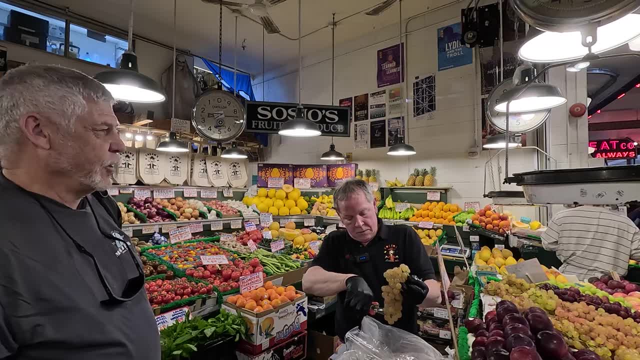 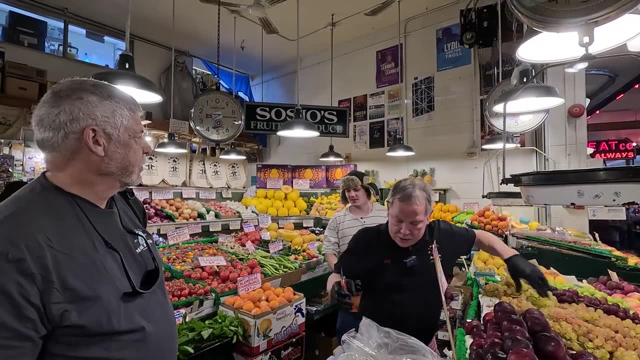 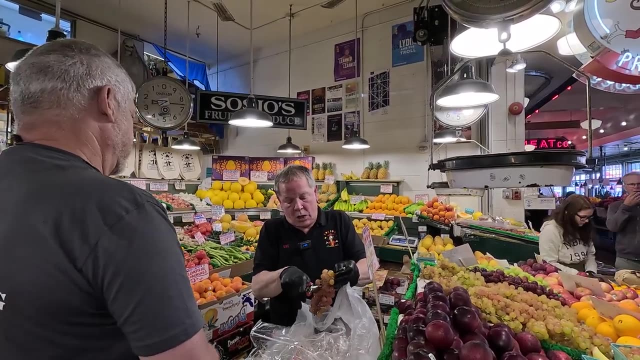 that we want, because every year there's less and less. well, you keep a pretty good secret on them, though, right um, I will put them on display, usually two or three times a year, but for the most part I'll sell 30 cases- 40 cases a week, if that's all I get um, without ever putting them. 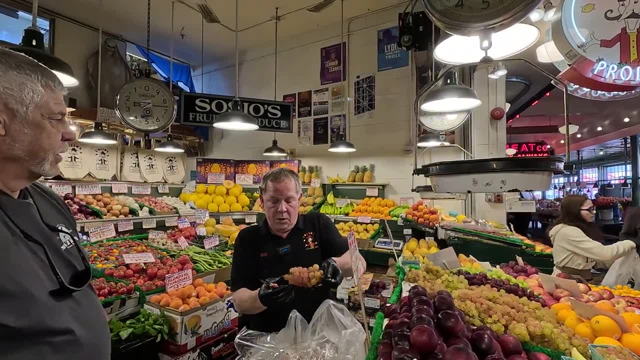 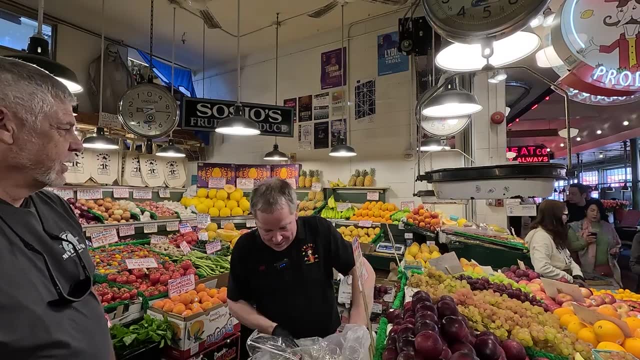 on display. yeah, yeah, people know to ask for them people that don't know. well, what you don't know, it doesn't hurt you, doesn't hurt you. yeah, I've been buying from you for a couple minutes 30 years now. yeah, that's only about half the time I've been here. so 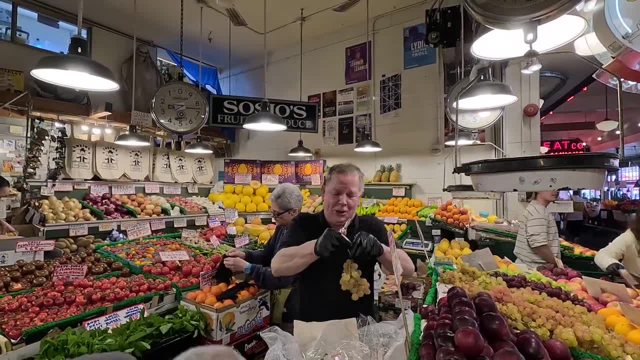 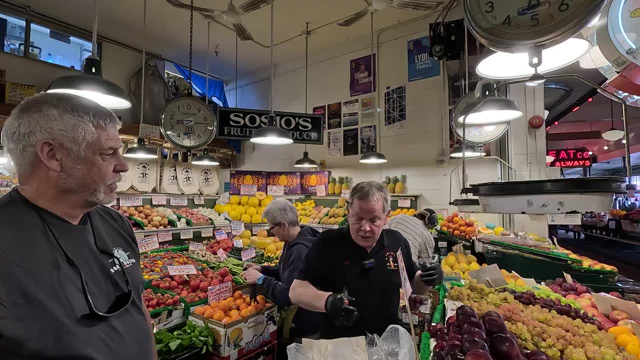 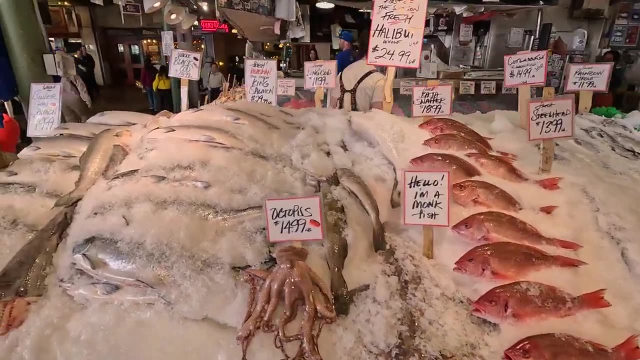 yeah, yeah, I'm ready to head out of this place, so hopefully soon. retirement is good when you decide to do it. well, I know I just need to have somebody that's coming, I mean somebody that's excited to buy this place. after you buy your veggies, and Mike strolled down to the Flying Fish to get the rest of dinner. 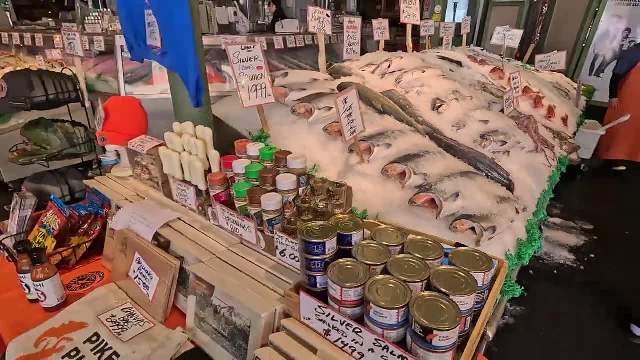 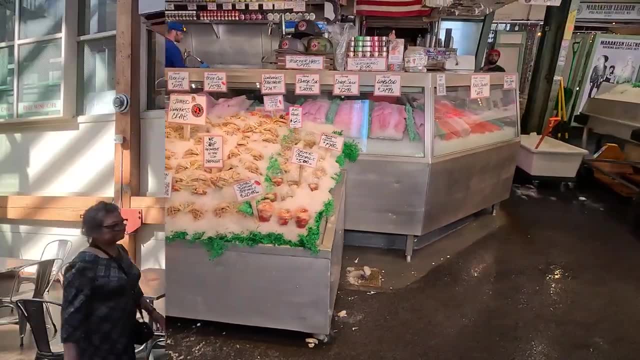 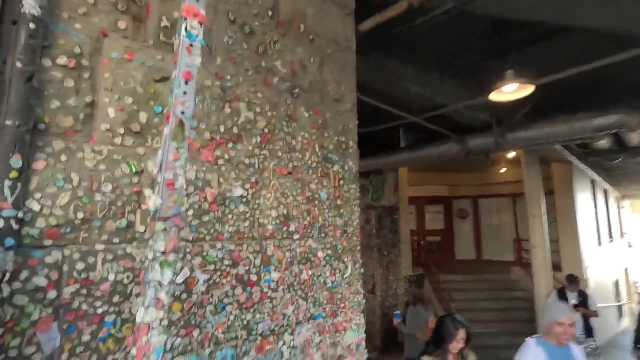 whether it's salmon, cod, crab, halibut, they'll pack it on ice for you to go. then it's on to look at the rest of iconic Seattle's Pike Place Market. no trip to the market would be complete without a stop at the iconic gum wall. 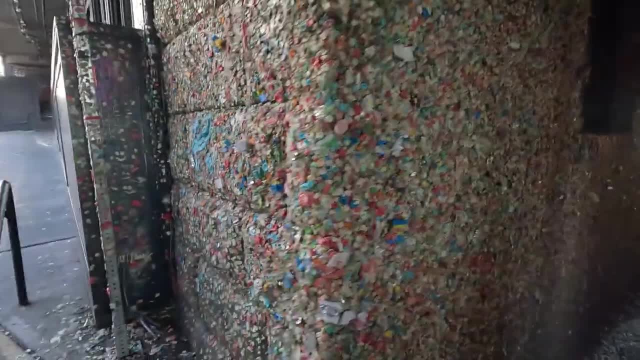 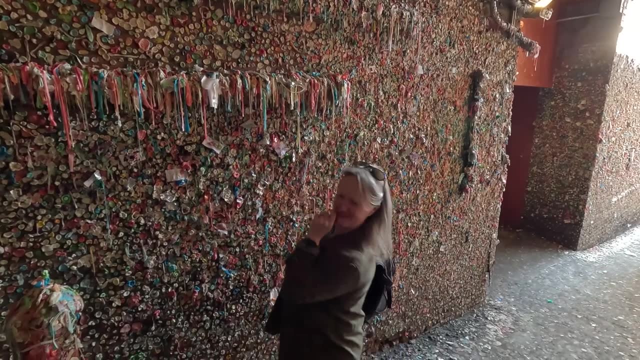 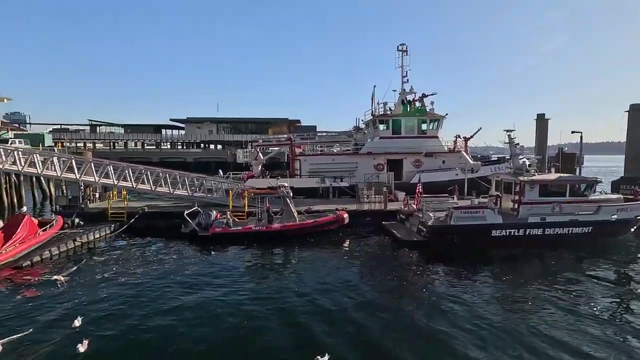 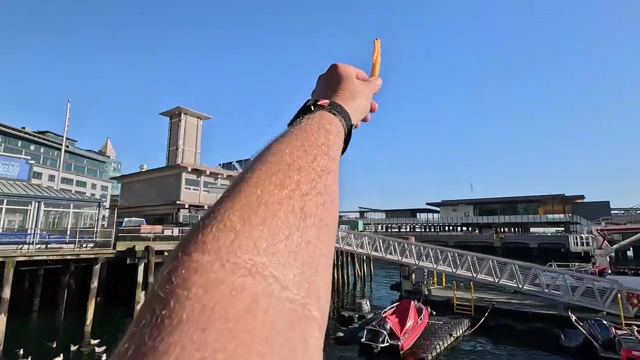 remember. you can leave it, but no sampling. after a quick run up to Top Pot Donuts, it's time to head back down towards the waterfront. check out fire station number five and the fireboats right next to Ivers Seafood Restaurant. grab an extra large order of fries and don't be afraid of overfeeding the seagulls- they're pretty. 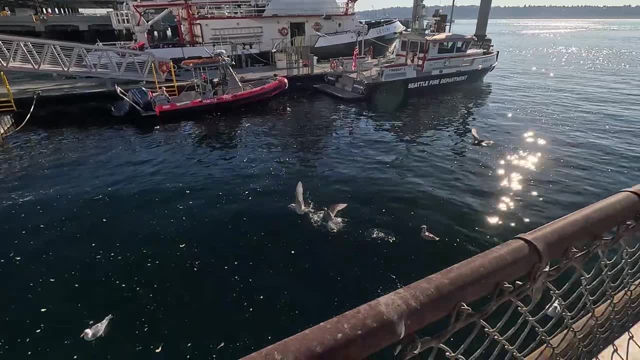 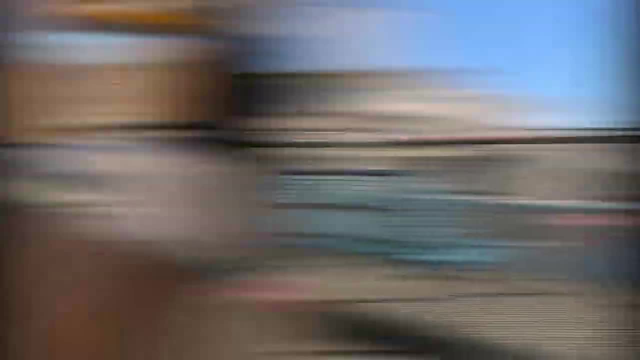 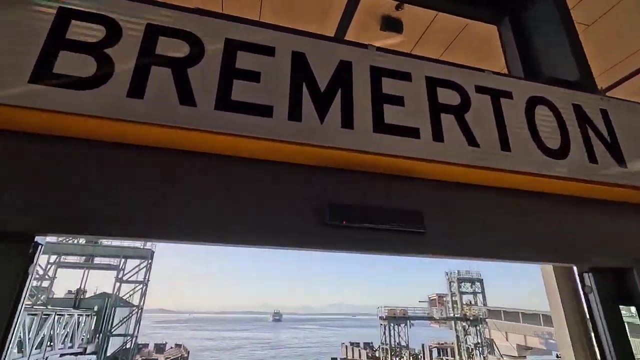 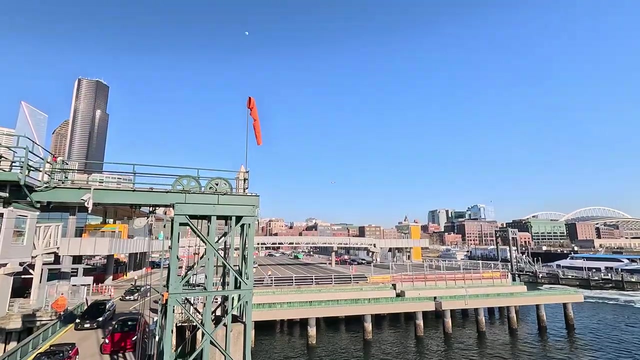 dainty eaters: two, two, two, two, two, two, three as you get ready to head back to Bremerton. buy your tickets, get in line a couple minutes early and then walk on from the upper deck. it's back across the sound. Seattle Washington is one of the most beautiful Skylines in all of the country. 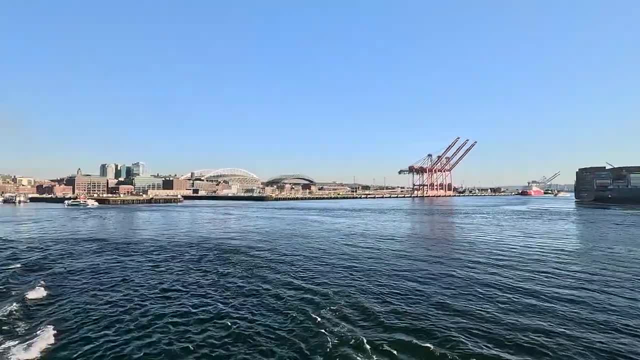 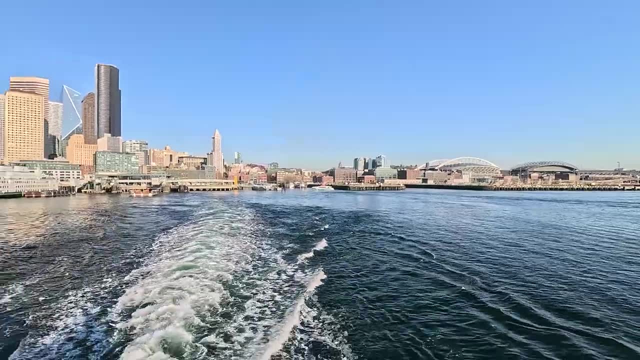 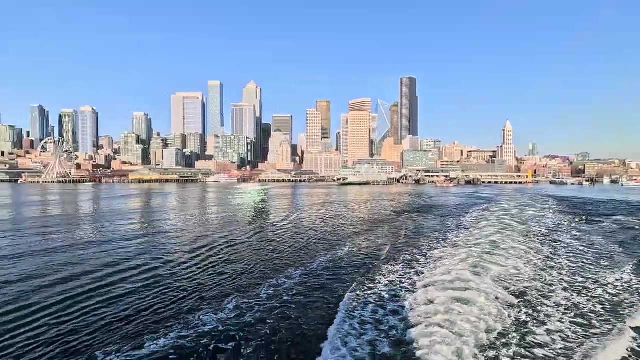 and watching it from the deck of a Washington State ferry as you leave Seattle is one of the most amazing views you'll ever get, from the sweeping views of T-Mobile Park, home of Seattle Mariners, to lumen field where the Seahawks play, all the way through downtown up to climate pledge arena where the Kraken play, and a space. 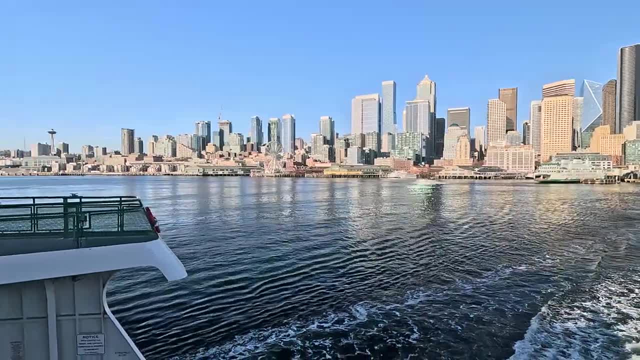 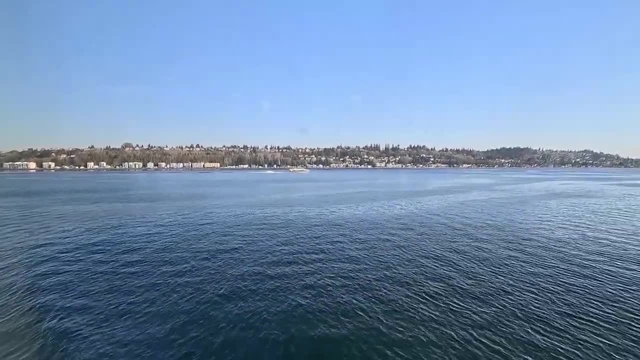 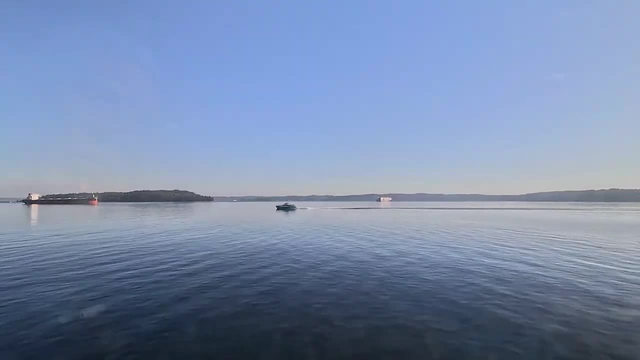 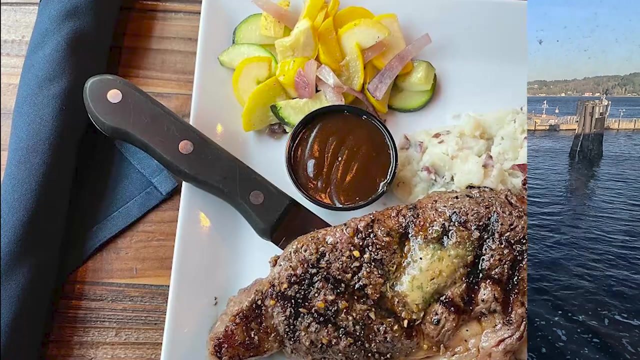 needle. it's just amazingly beautiful. sit back on the hour-long crossing and enjoy the views. when you arrive back in Bremerton, there's still one stop left to make the axe and arrow. it's owned by two army green berets and a fire captain, so you 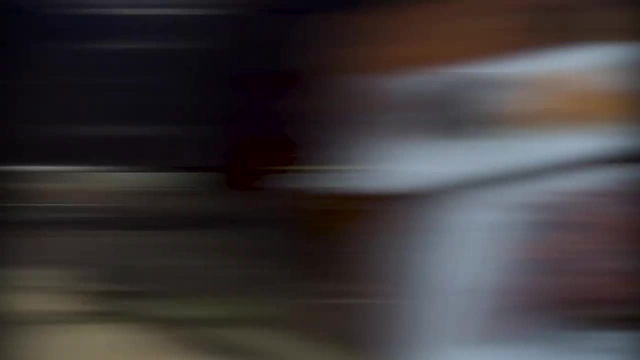 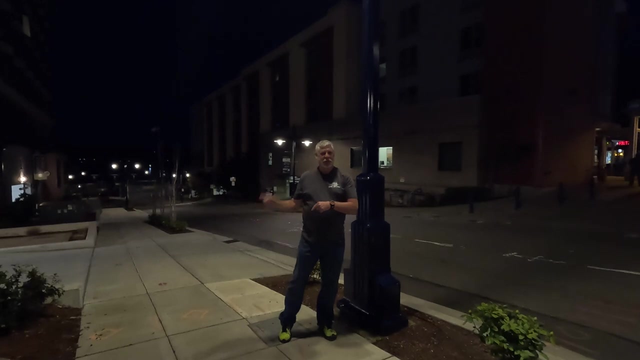 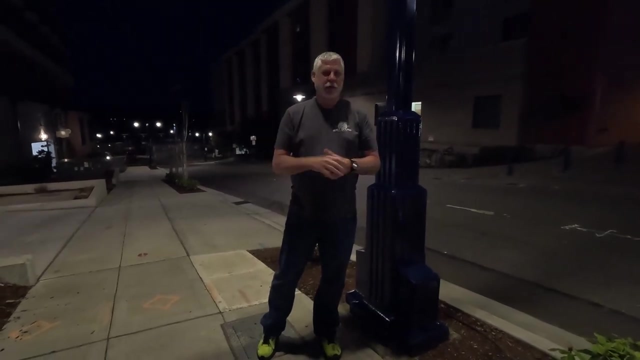 know the food and drink are outstanding. all right, so a full day, Bremerton over to Seattle. walk through the Pike Place market, talk to some friends that we knew from years and years. back bought some veggies and some fruits, ate our way through the market back over to Bremerton, had dinner, maybe an adult beverage, and it's time to.